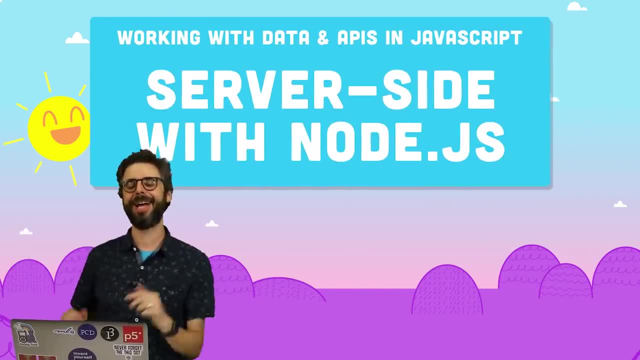 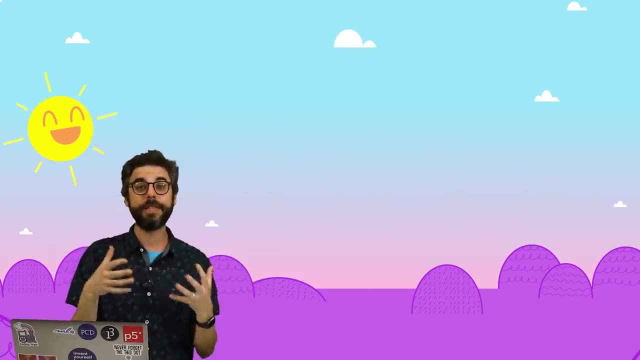 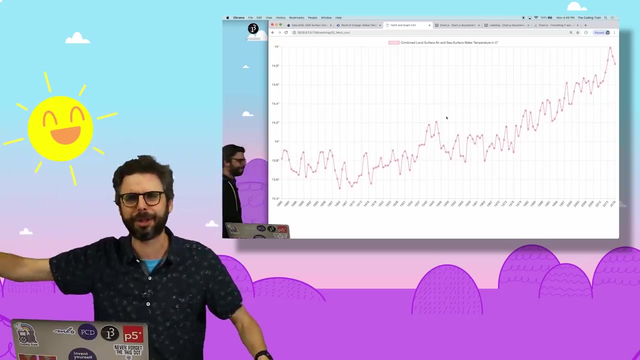 Welcome back. It is time for module two, And in this module I'm going to do something quite exciting and quite different than what I've done so far. Everything that I did in the previous example, it was all client-side JavaScript: Drawing the map, graphing the global temperature data, loading images and displaying them on the web page with the fetch function. 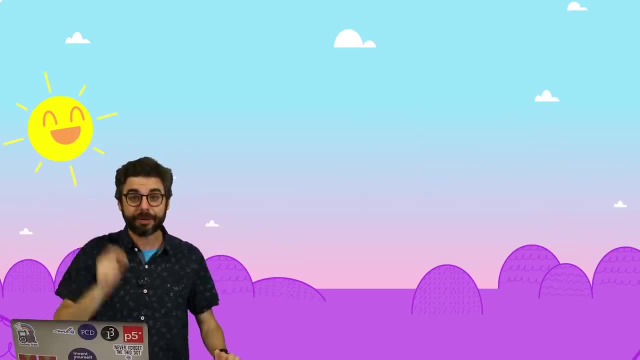 All of that was done with client-side JavaScript, meaning JavaScript written into the HTML page itself. But there are a lot of things that you, that I, that the people of the world who are doing this programming thing, want to do- working with data and APIs- that you cannot do with client-side JavaScript only. 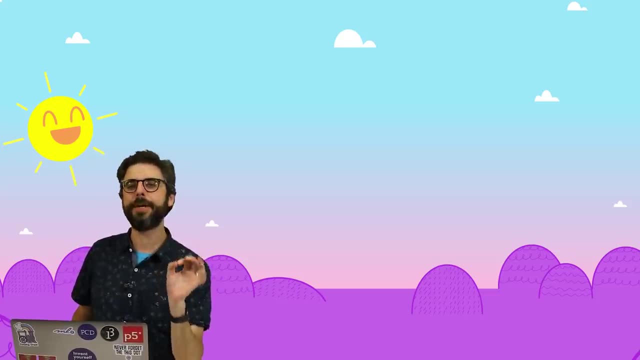 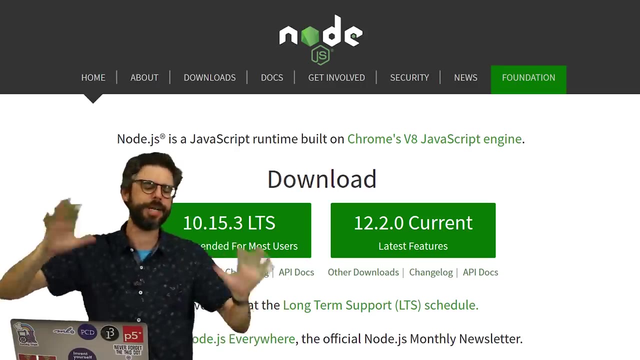 So in this module, I'm going to show you server-side programming, And I'm going to use a JavaScript runtime called nodejs, which can be used for server-side programming. Now, the details of what server-side programming is and how I'm going to do it, that's to come. 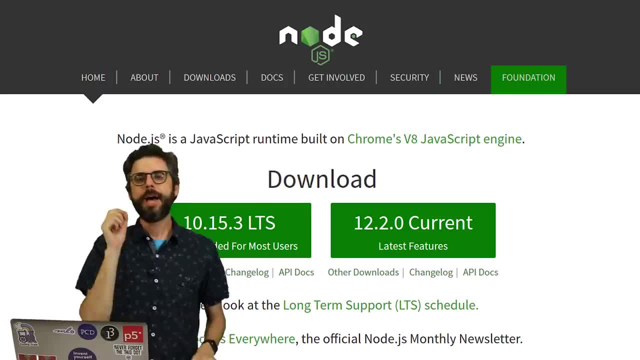 But this project that I'm going to build, the fundamental thing, the reason why we need node for this project, is for data persistence. I want to gather some data and save it and get it back later, And this is not something that you can easily do without writing a server. You can certainly use somebody else's server. There's something called database as a service where I can just say, hey, you've got a server, can I sign up for you and take my data? And then, like, I'll ask for it back later. 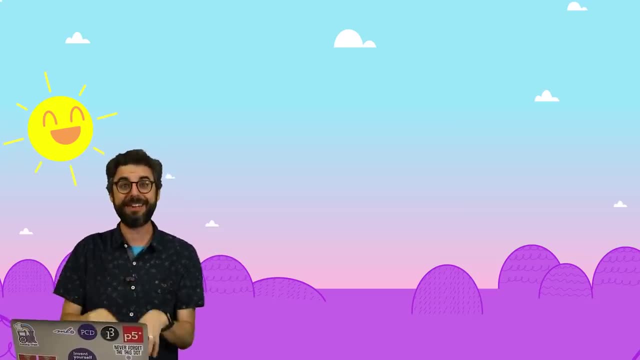 But I'm actually going to create a server that's going to run on this laptop here And I'm going to save the data here. Now, at some point, I'm also going to need to show you how to get that server to run somewhere else besides your own laptop. 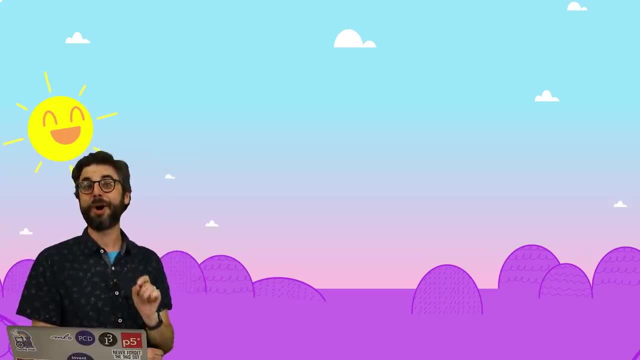 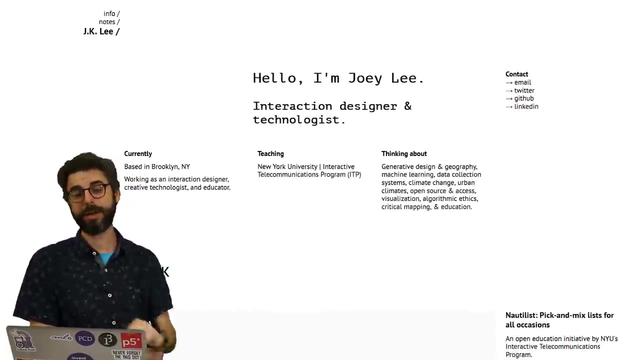 But that's a place to start. The project that I'm going to build in this module is called the Data Selfie App, And the Data Selfie App is an example project by Joey Lee, who's a designer and researcher. He teaches a class right here at NYU, at ITP, called Quantumness. 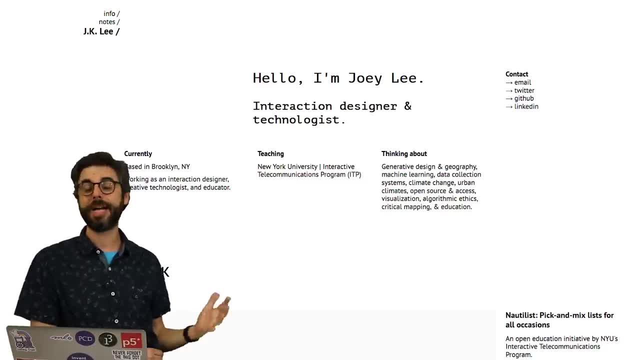 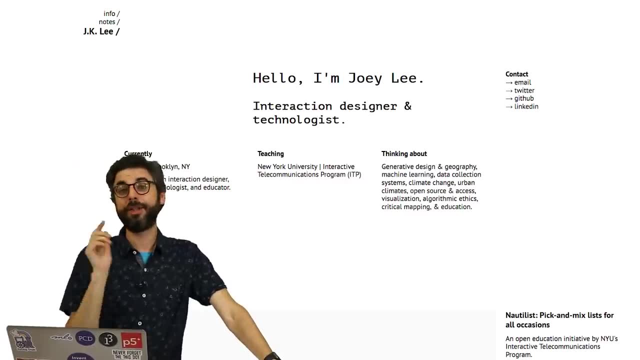 It's about data and self-tracking, And so Joey has graciously given permission to use to build on top of his examples as part of this series. In this video's description, I'll link to Joey's website so you can learn more about his work. 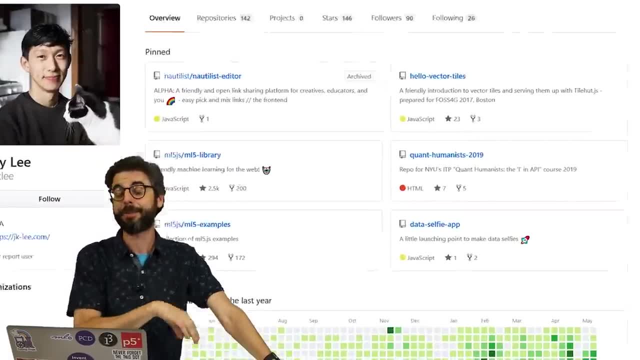 as well as to the original GitHub repo for the Data Selfie App, so you can find all of the code for the things that I'm going to show you Now in order to follow along with the code that I'm going to write and demonstrate as I build this project. 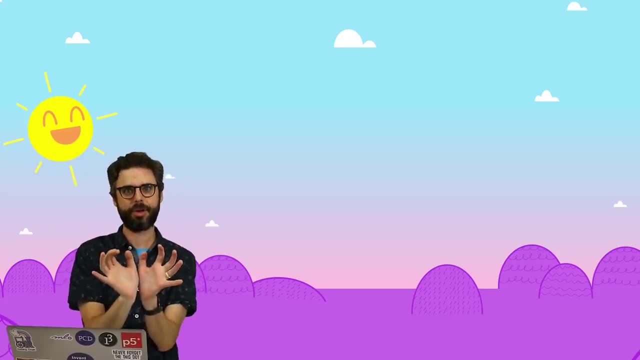 you're going to need to download and install some stuff that you might not have on your computer already. It's going to be confusing, because you might be using Windows or you might be using Mac, and I'm using a Mac and oi. how are we going to solve this? 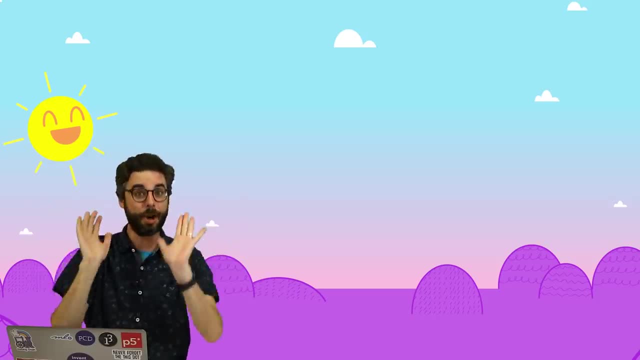 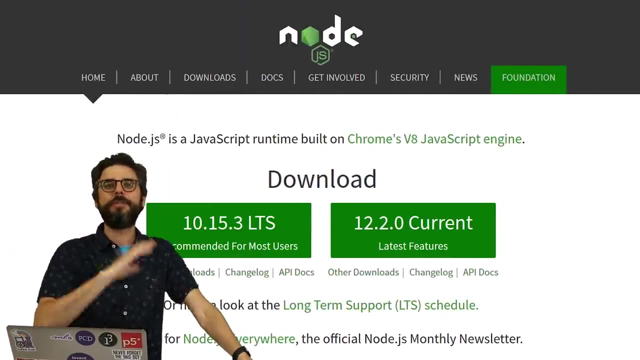 All right. So let me give you a list of the things you need and help you with some resources to find those things. Number one: you need to install Nodejs. That should be as easy as going to nodejsorg and following the installation instructions for your operating system. 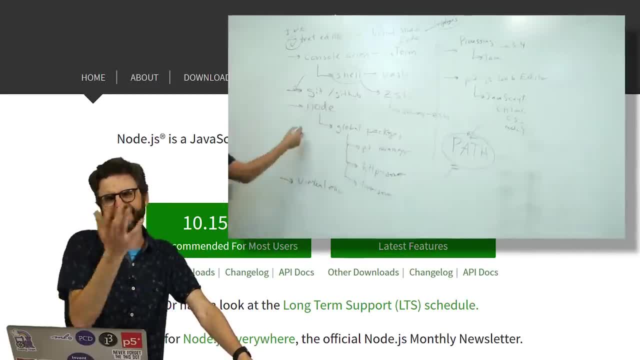 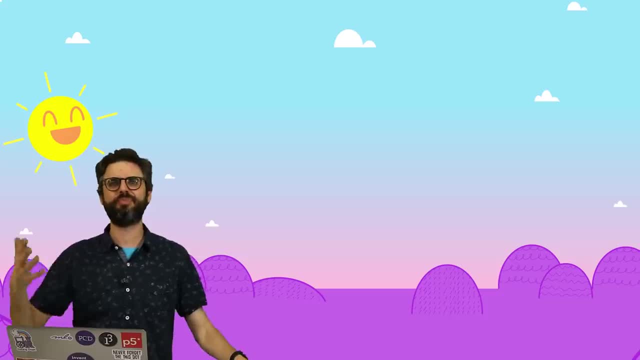 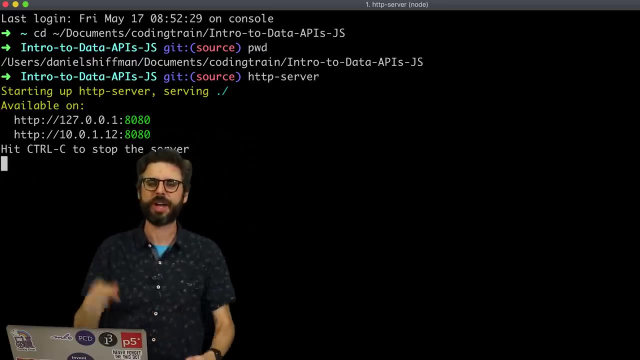 I do also have an entire video about downloading and installing Node and what Node is that I'll also link you to if you want more background there. You're also going to want some kind of console application, some command line, terminal thing that you can open up and type commands in to run Node stuff on your computer. 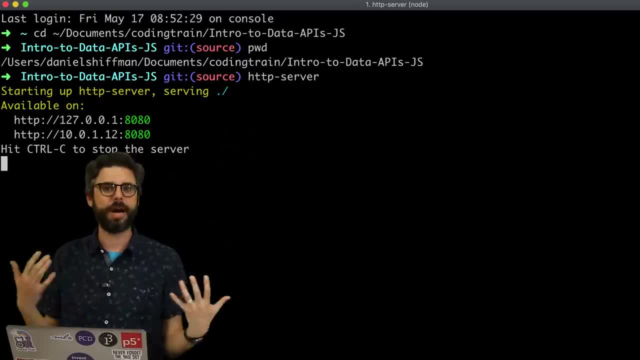 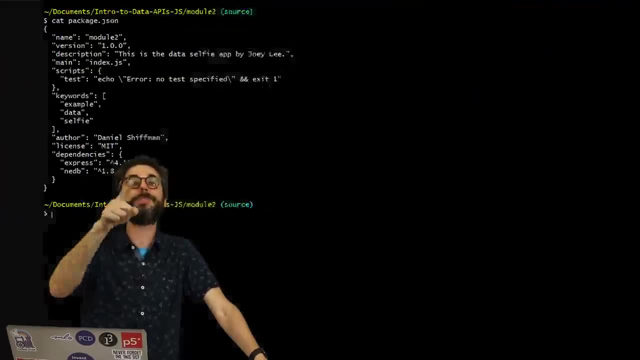 I'm using iTerm, which is an alternative to the Mac's built-in terminal application. On Windows, I hear people like PowerShell, just the built-in command thing. Oh, and Git Bash. Git Bash is possibly a good one too. 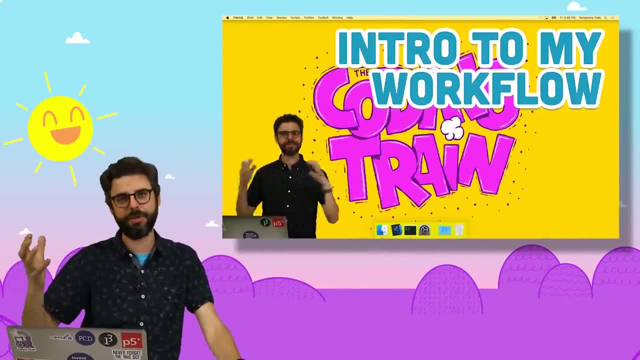 I actually have a whole workflow series where I go through all these bits and pieces of everything you need to have your environment set up to follow along with what I'm doing, So you can also just go and find that series, watch that and come back here. 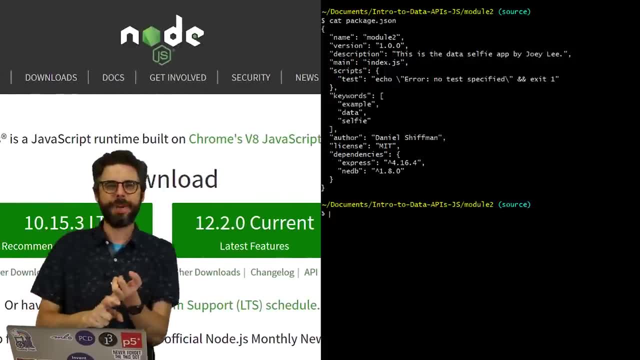 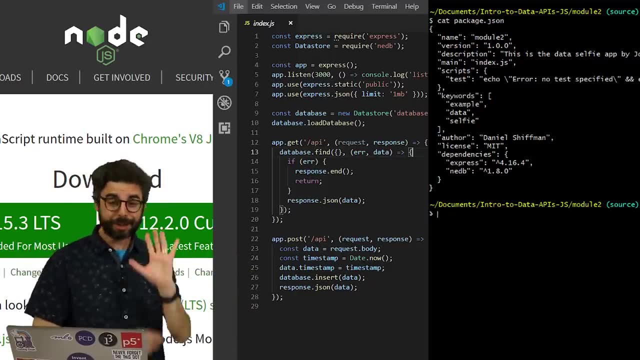 But all you need is download Node, you need some kind of shell command prompt thing and you need a code editor. If you've got that, you're ready to go. So before I get to coding and building the actual project, let's just talk for a second about what is Node. 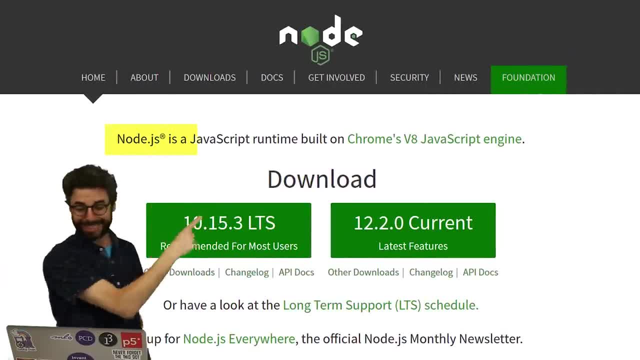 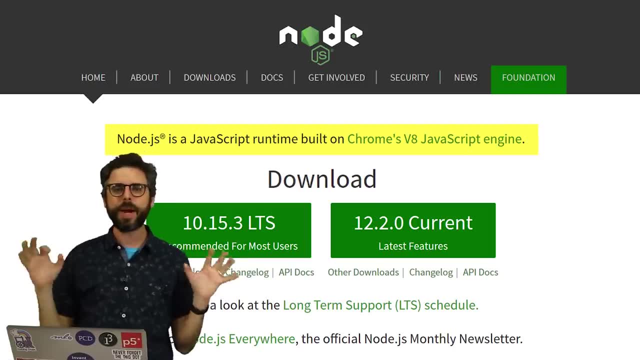 Now, if you go to the Node website, it says right there, Nodejs is a JavaScript runtime built on Chrome's V8 JavaScript engine. Whew, that is a mouthful. Let's try to understand what that is. What do I mean by runtime? 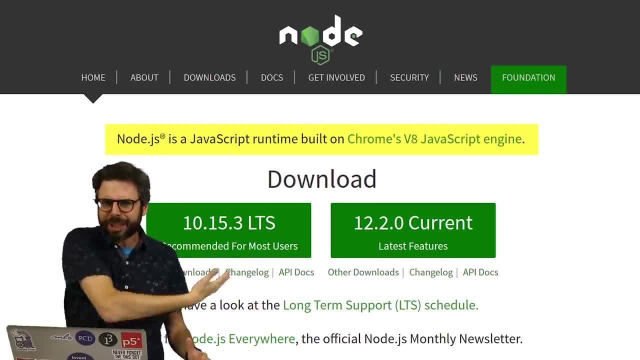 So normally when I'm typing JavaScript I'm executing that stuff in the browser. The JavaScript has no meaning without the browser itself. Suddenly, with Node I can start to write JavaScript without the browser. It's its own runtime. The code runs on your computer. 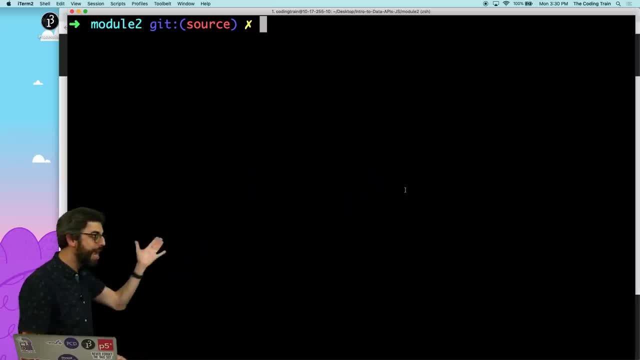 Let's look at what that means more practically speaking. So here I am with my command prompt. It's a command line access where I can type in commands. So hopefully you're here, you've downloaded your terminal app thingy, you've got it going and you've installed Node. 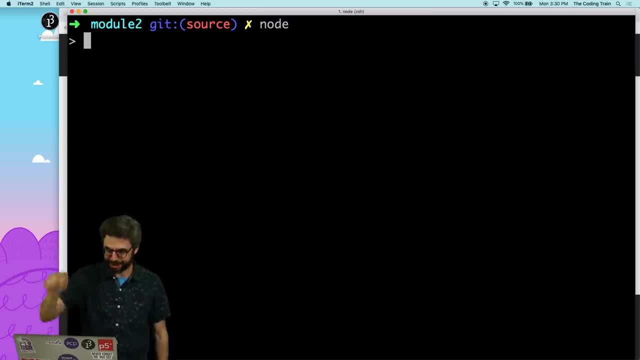 If I now type in N-O-D-E Node and hit enter, suddenly I have entered the JavaScript runtime. This is very similar to like the developer's console in the browser, But here I can start typing in some JavaScript stuff like const x equals 5.. 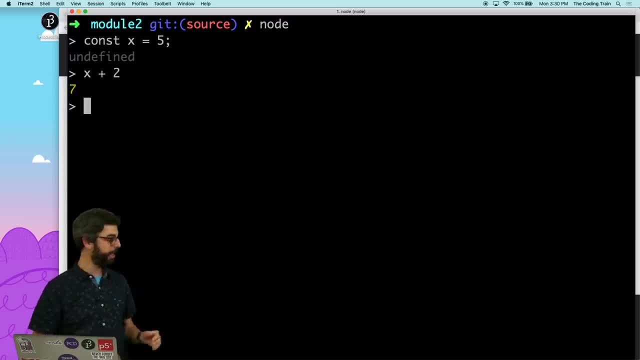 And then I can say x plus 2. And it's going to give me the number 7.. So we can see this is a runtime and I can write JavaScript and run JavaScript. Now, this is not typically how you would use Node. 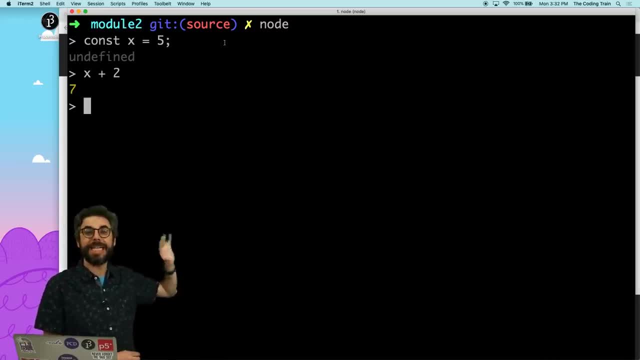 Typically I wouldn't just be writing a lot of code just line by line in my terminal itself. I would write a bunch of JavaScript code in a JavaScript file and then execute it through a Node command. So let's see how that works. So I actually have a file called indexjs. 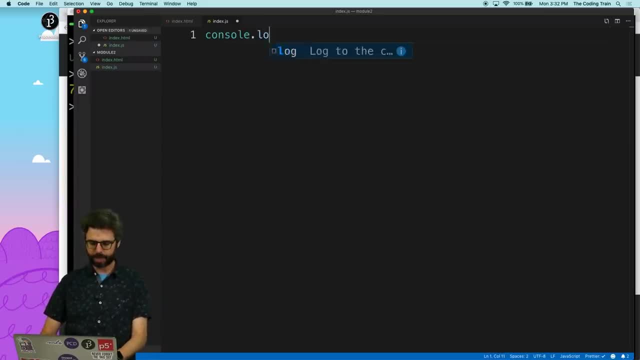 It's just a JavaScript file And I could put something in like consolelog hello. And I could say: const x equals 5. And I could say something like you know, consolelog x plus 2. And let's see what happens. 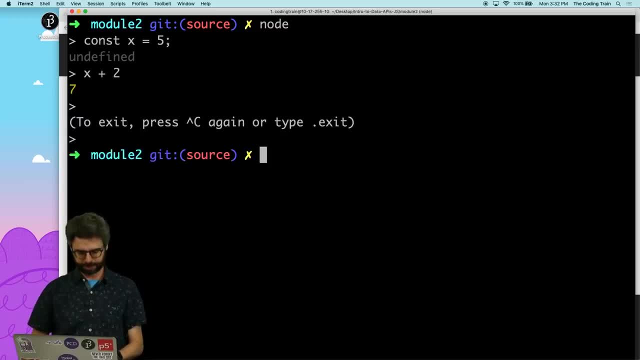 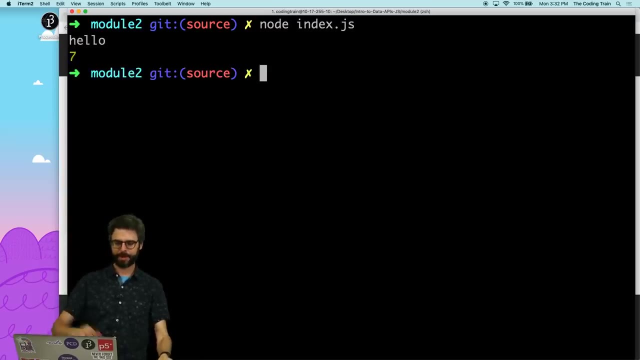 So now, if I go back to the terminal, I can type node indexjs. And this is me saying hey, execute the code line by line, in the order that it's written, of what you find in that file. So I'm going to do that right now. 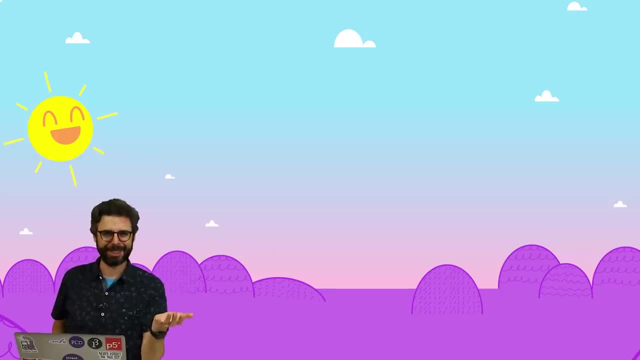 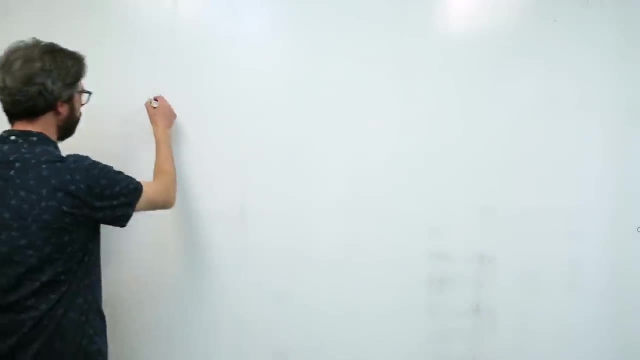 And there we go. So what is it that I want to write in that indexjs file? It's clearly like console logging a bunch of things. I can see that it works, But why am I using Node? The reason why I'm using Node is that I want to create a server. 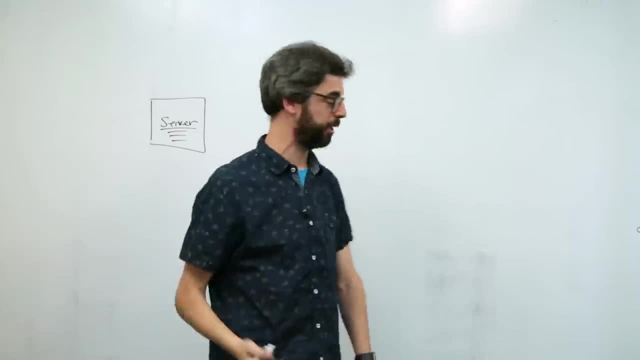 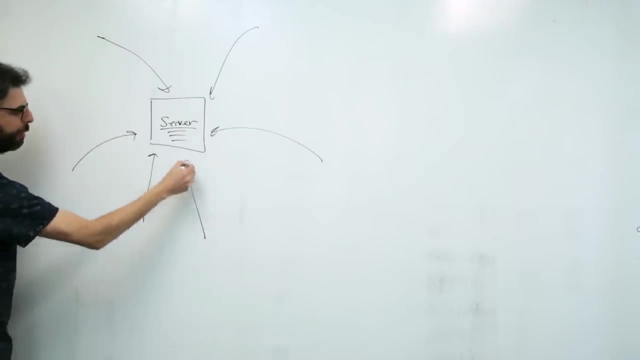 A server is an application that runs and listens, And what it listens for is it listens for requests, people who want to connect to that server. So this server is going to be the central repository of the data of my application, All of the different clients. 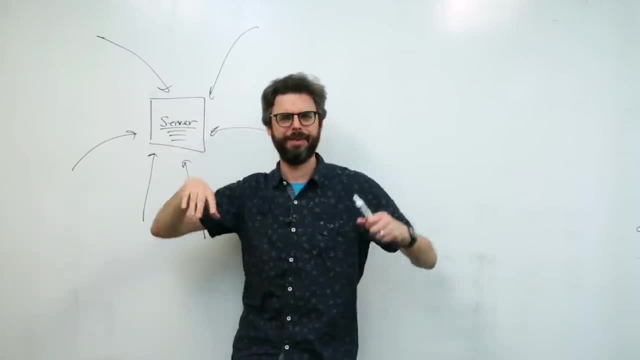 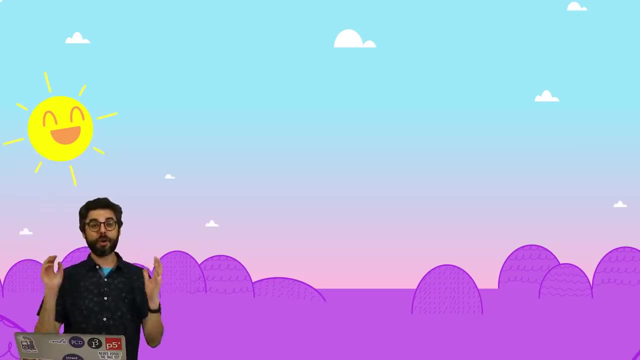 whether it's you on your phone or so-and-so on their laptop or somebody else on their internet connected toaster, make a request to the server and grab some data. So I could come back over here and just start writing. I could Google, write a web server with Nodejs. 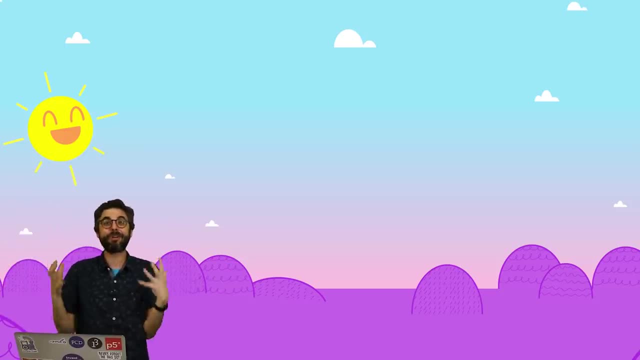 I could find some code, I could start typing it in there And I could create that server. It's going to open up a connection and start listening. However, one of the ways that is very typical when working with Node is to find a package. 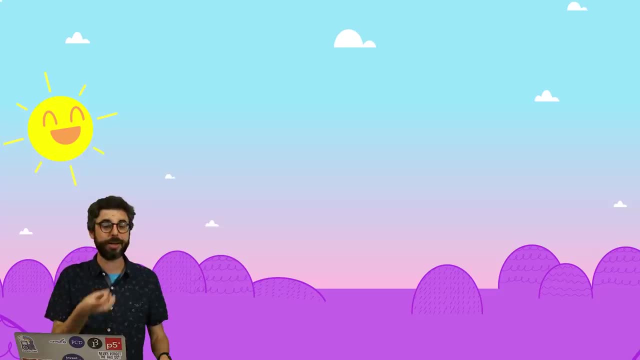 a Node package that has some of the functionality you're looking for. install that package- It's like a library or an add-on- and make use of that functionality. And the Node package that I want to use to create my web server is something called Express. 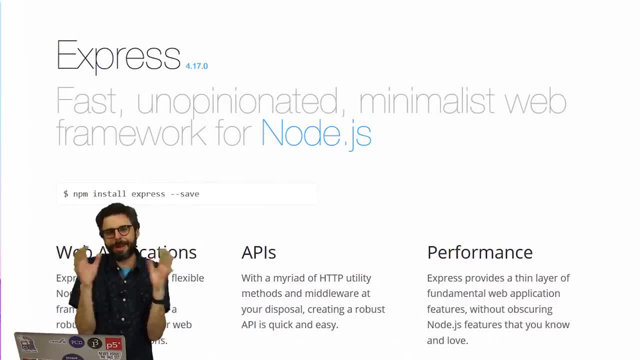 Express is a pretty minimal and very simple framework for making web servers And it has the core functionality you need without a lot of bells and whistles, So we can kind of get up and running with it really quickly. So now we have Node. 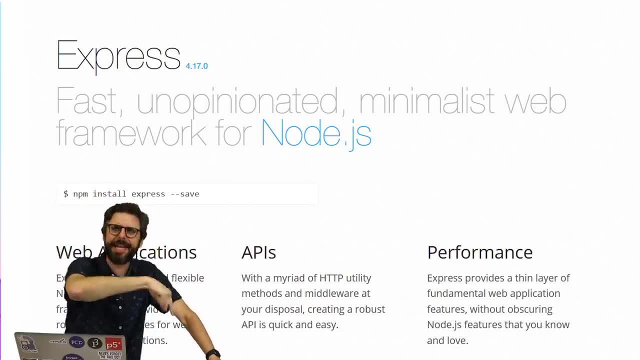 We can write JavaScript code in a thing and run it with Node. So in theory we could write some JavaScript code to make a server. but we need this package. How do we have access to the Node package Express in our Node code? Well, there's a package for NodePackageManager. 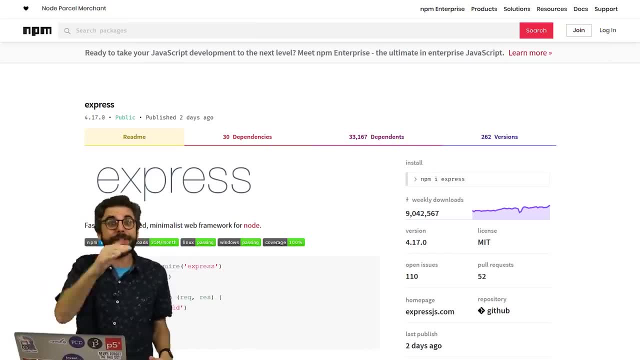 and it's a thing that manages all of our Node packages for us. You don't have to install that. In fact, when you installed Node, you also installed NPM- NodePackageManager. If I want to use NPM with this project, 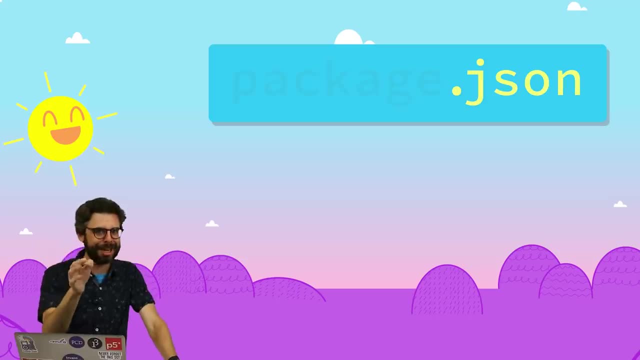 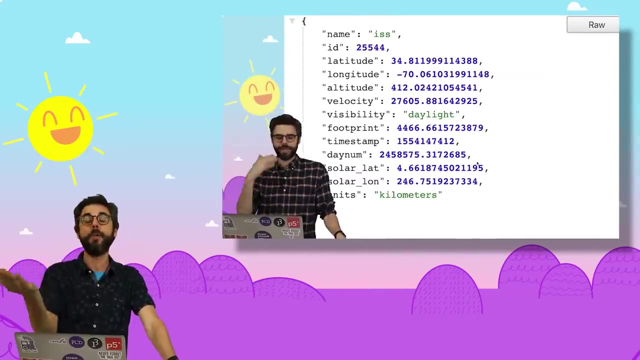 I need packagejson. The good news for you is that json in packagejson. You know what JSON is because we've worked with it. We have gotten data in JSON format- JavaScript object notation- before in previous examples. Packagejson is a special kind of file. 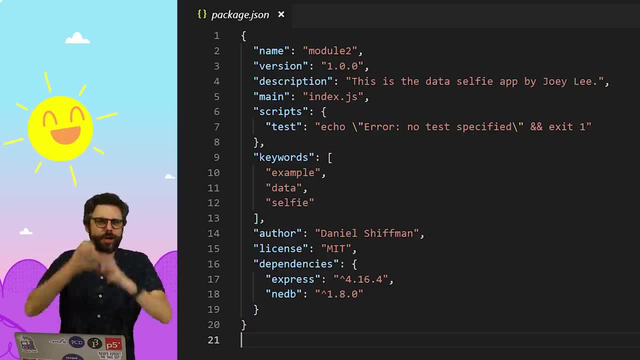 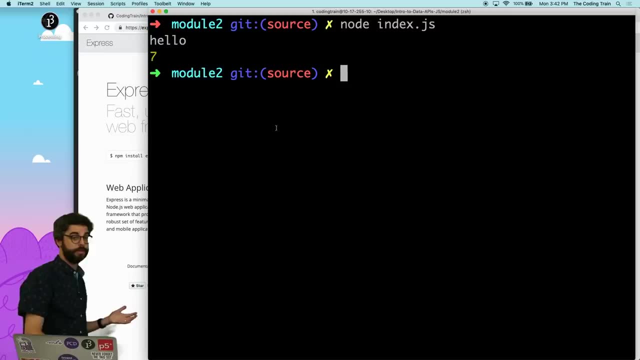 This is where all the meta information about our project, what Node packages we're using, what our project is called- And by project I mean web application- All of that's going to be in packagejson. To create the packagejson file: 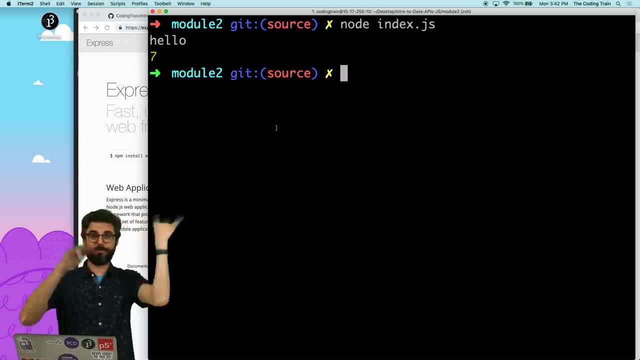 I could, if I want, just make a file called packagejson and type some stuff into it. but if I want to not make any mistakes, if I want to be sure, there's a nice command line utility from NPM itself that will generate the file for me. 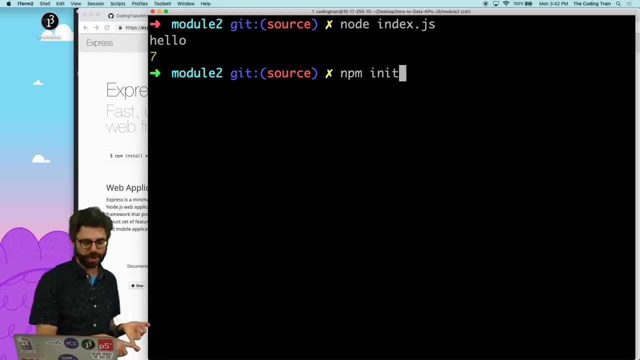 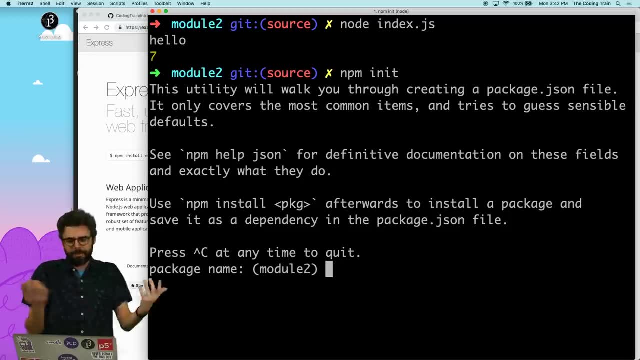 And that is npm init. So as long as I've got Node installed, if I'm in the project directory, I've got packagejson in it and it's going to walk me through what I need in the packagejson file. So one thing is I need a name. 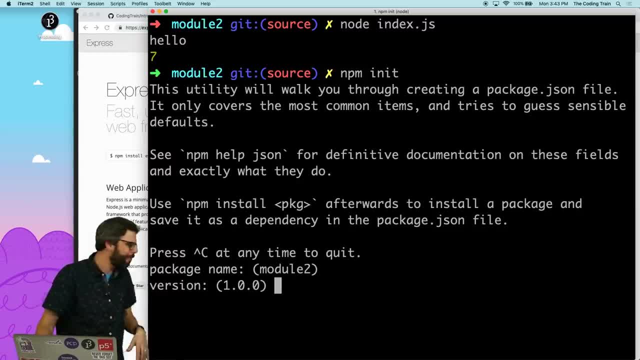 It's giving me it's guessing, because the folder is called module two. Module two, that sounds good. I'll just hit enter Version number. I'm not going to worry about the version number. This is important if I'm building an open source library. 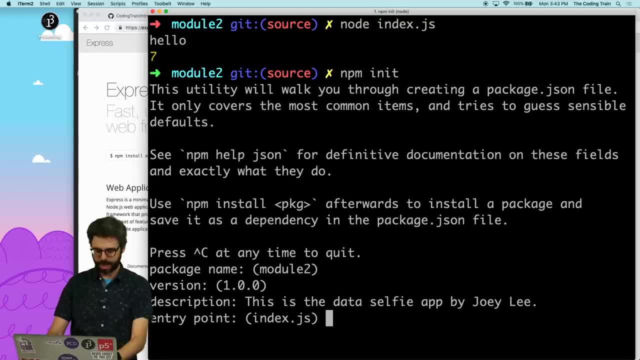 I need to really keep track of version numbers, but I'm just kind of tinkering around here. Description. let me add something. This is the data selfie app by Joey Lee. I put my code in that I want to run when I want to run this project. 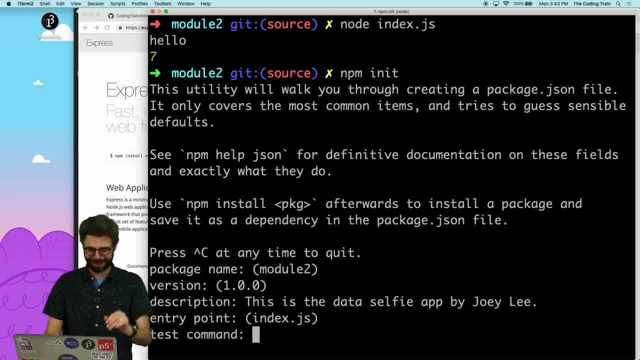 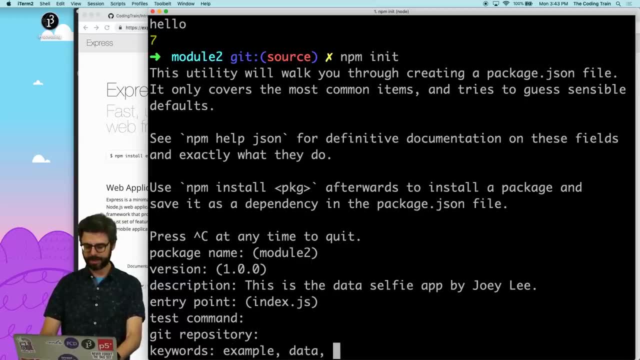 Test command: I'm not worrying about testing right now. I'll refer you to some other videos about that, if you're interested. Git repository: I'm not worrying about that. Keywords, example: data, selfie, something like that. I think I can give some keywords separated by commas. 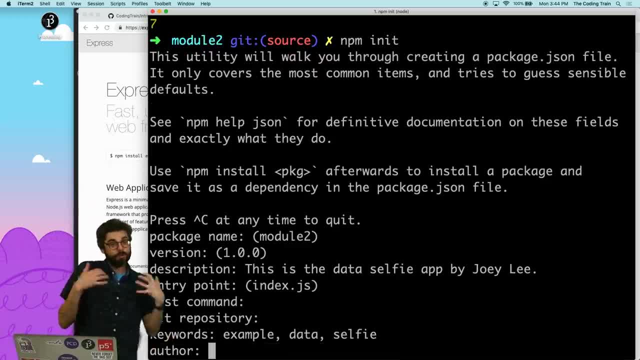 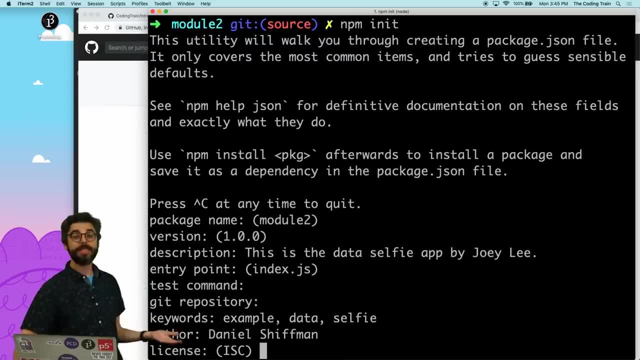 Author. this is a tricky one because I'm basing my work off of Joey's work. I'll put my name in there for right now and I'll make sure that everything is well documented of where it's coming from as I go. License I'm going to put in. 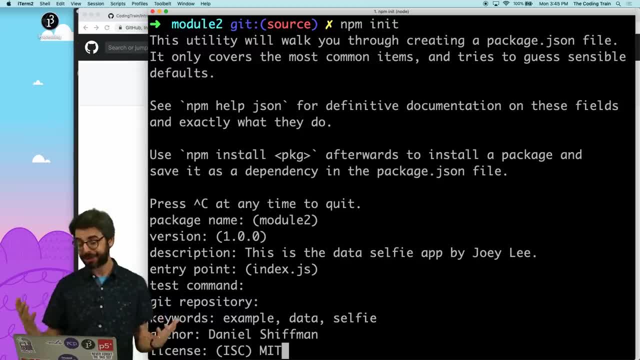 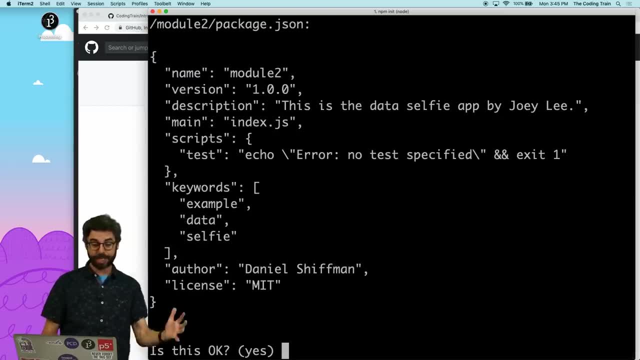 MIT. That's a very permissive license that basically lets you do just about anything you want with the code. That's the same. I'm using the same license that Joey is using And then look at this it's giving me. this is the information that is going. 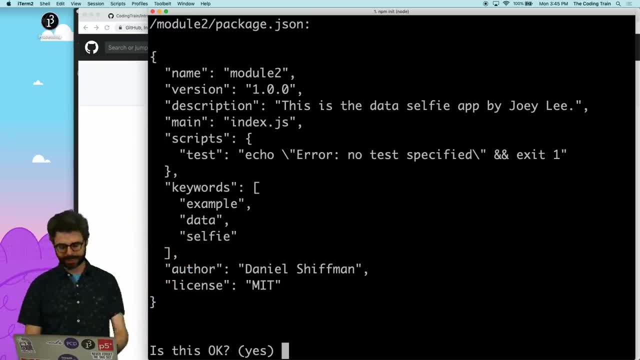 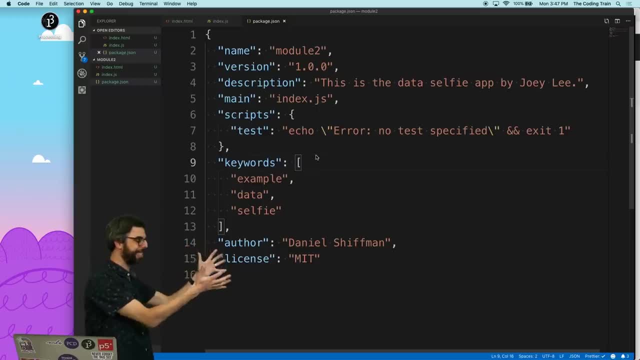 in that packagejson file. Does it look okay to me? It does. I'm going to type yes. If I go back to my code editor I can see there we go. here's the packagejson file. All the information that's needed is in there. 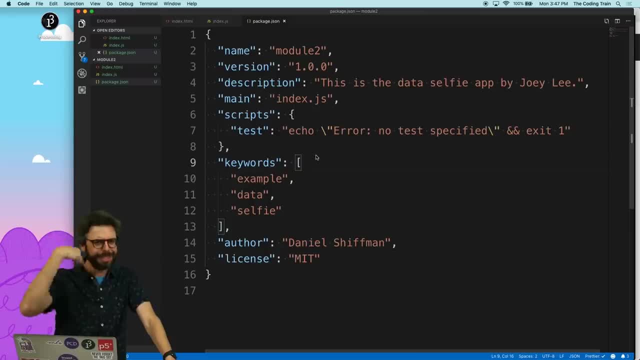 It's formatted correctly. I'm ready to go, But I'm not ready to go right. I'm not doing this in the first place. I'm trying to get to the point where I can install the node package express, The web framework I want to use. 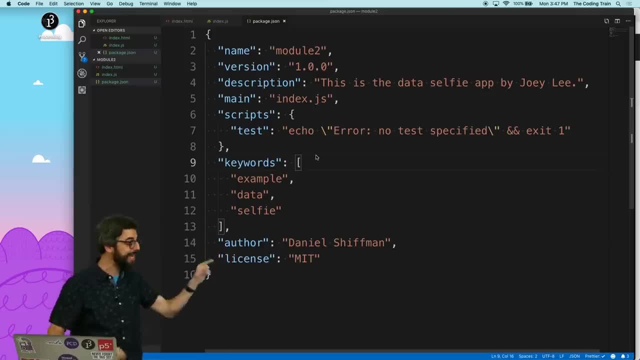 for creating my server. The reason why I need this packagejson file is in. this file is where I need to make reference to express. I need to say express is a package that I'm using for my project, But I don't want to edit this file directly. 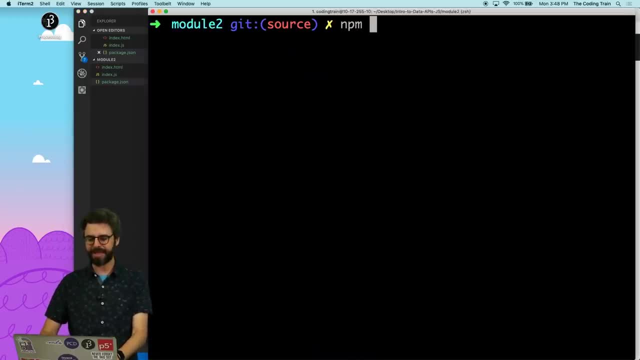 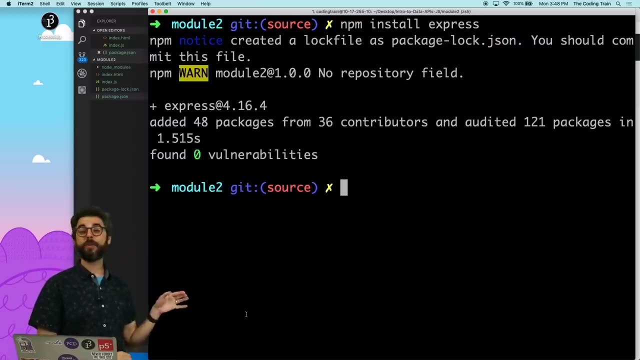 even though I could, What I want to do instead is: say npm, install express. Say npm, install express and run that. Once I've run this, two things are going to happen. Number one is we're going to see express pop up in packagejson. 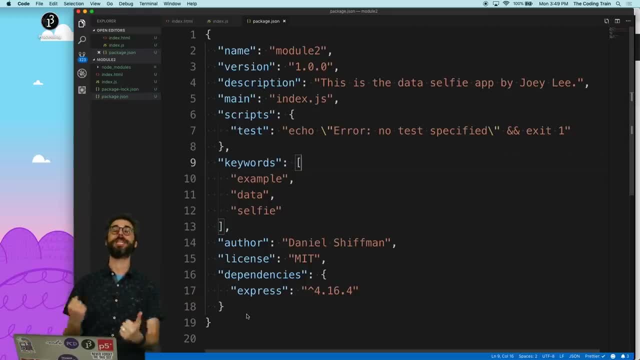 as one of the dependencies. It's a dependency of this project. My project depends on the existence of the express node package, which I intend to use quite a bit in this code. Other thing that's happened is I have a new folder called node modules. 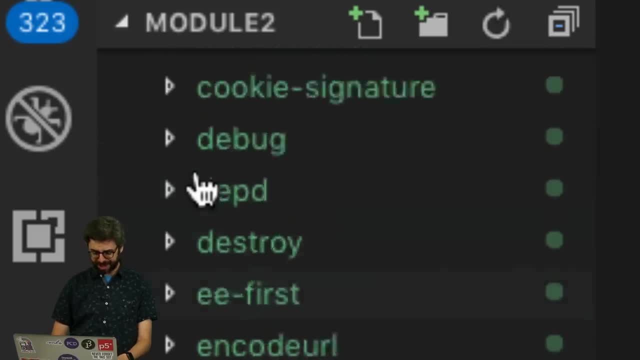 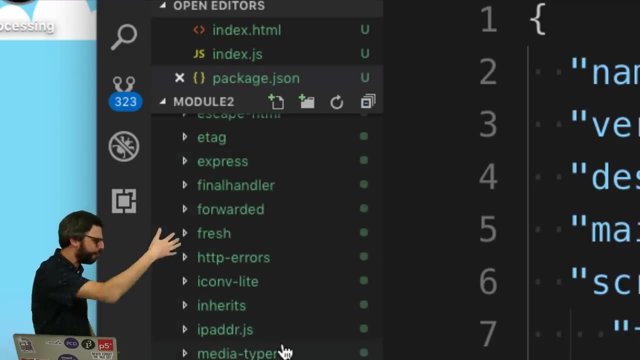 And when I look into this folder, there's so much stuff in here. So this is the thing. Oh look, there's express. I only said express, npm, install express. I didn't say inherits or fresh or hdbrs. It so happens that most node packages 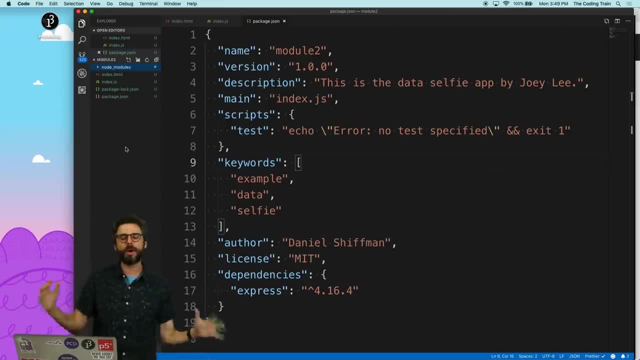 depend on other packages, and the node package manager is smart enough to know that if I'm saying install express, it's going to go grab everything else that it needs as well. So the nice thing is we don't have to manage that folder. Everything that we need will be in there. 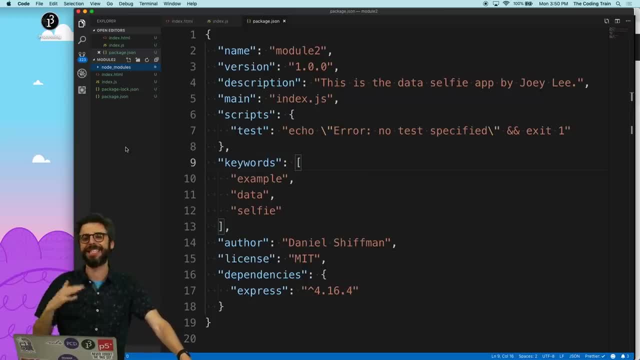 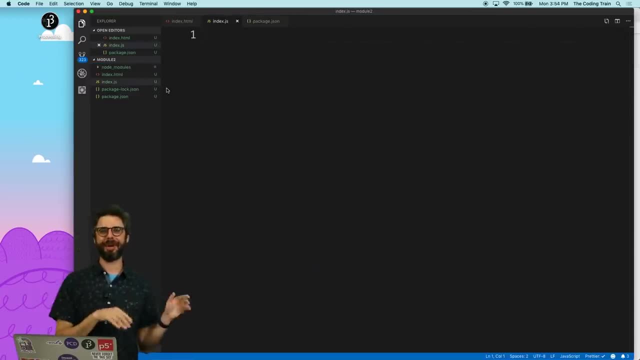 But don't be freaked out if you see all sorts of other things in there that you didn't think that you installed. They're coming along for the ride with express itself, Ready to write some code. So, in order to have access to the express package, 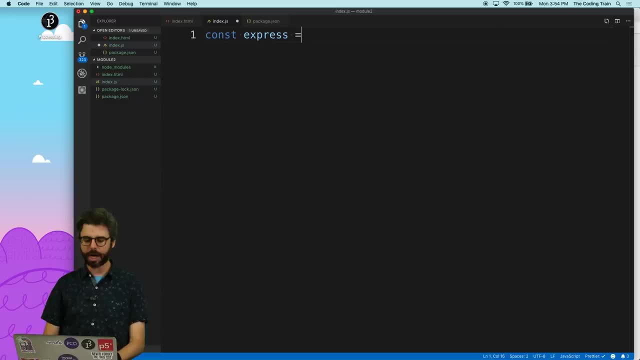 the node package express. I need to use require So I can say: const express equals, require express. This is basically like an import statement. Hey, you know that node package I installed called express. Give me that thing and put it all in this variable called express. 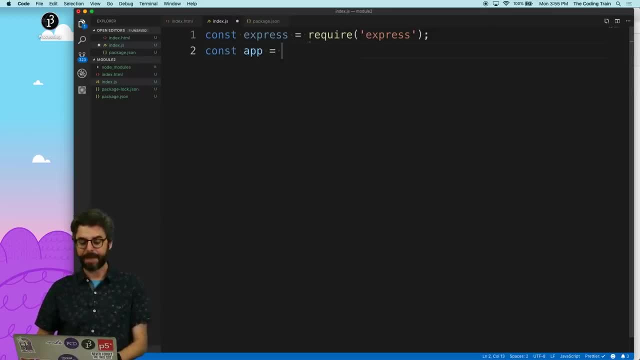 The reason why I want to do that is I want to create a web application. I'm going to call it app And the way I'm going to create that is just call the express function, So that whole library, the whole node package express. 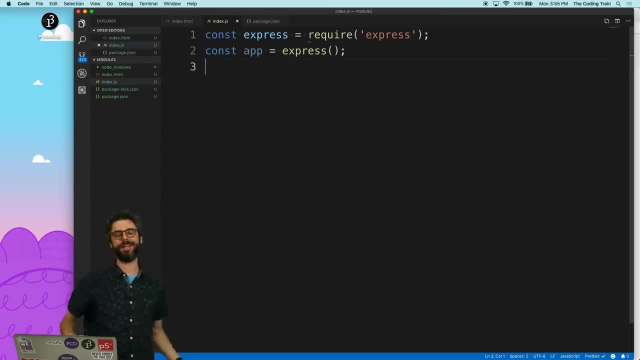 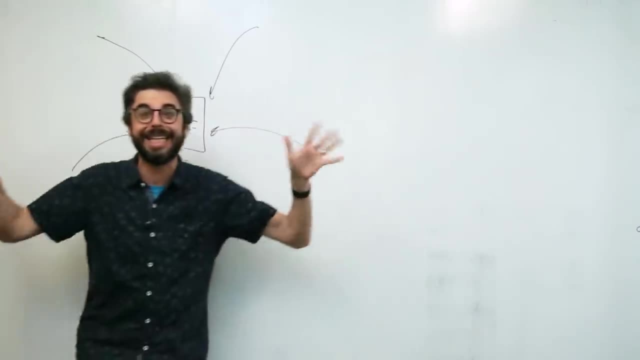 basically comes in as a big function that I can just execute and put in a variable. The first thing that I want to do in a web server. if I think back to my silly little diagram, here's the web server. It's listening, listening. Anybody want to connect to me? 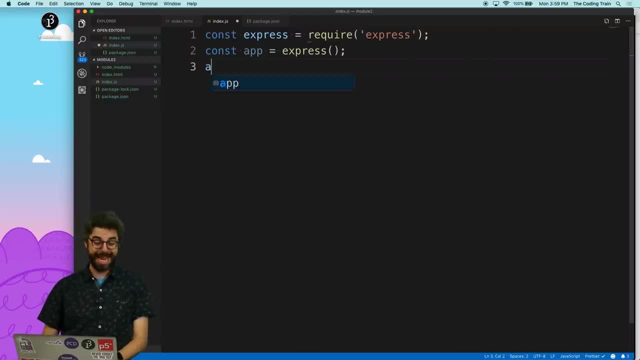 is, I need to start listening. So now I can listen. I can just actually say applisten. And when I want to start listening, I need to also specify something known as a port. Look at this, It's even telling me right here in node. 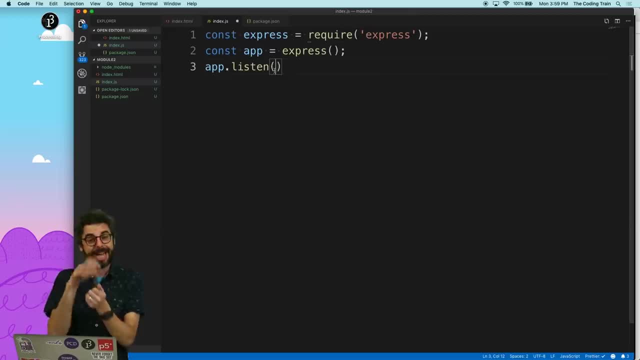 what I need The port is a unique number. It's like a numeric address at which I'm going to listen, So you could have different servers running different ports reserved for certain things. but it's beyond the scope of what I'm doing right here. I'm just going to pick some. 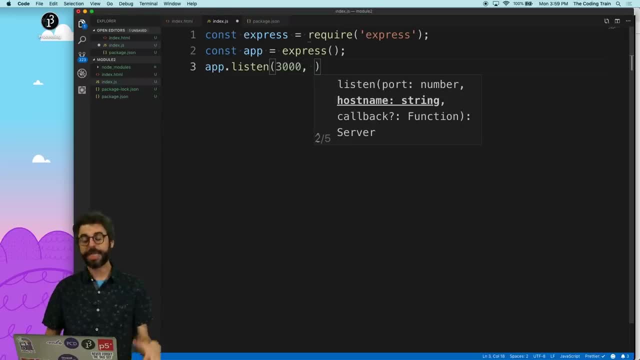 port that I know won't be used by something else like 3000.. And then I'm going to give a callback function here which basically is like just the callback that happens once the server is listening. So I'll use my arrow syntax and just say consolelog. 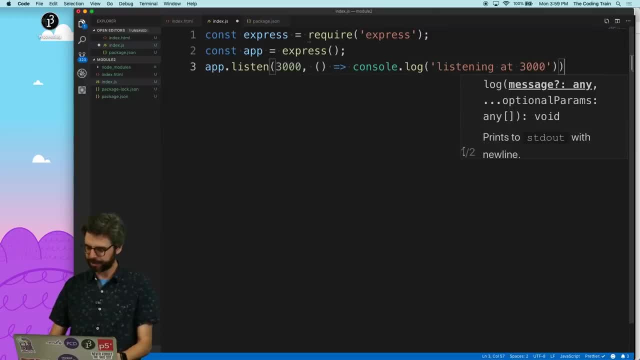 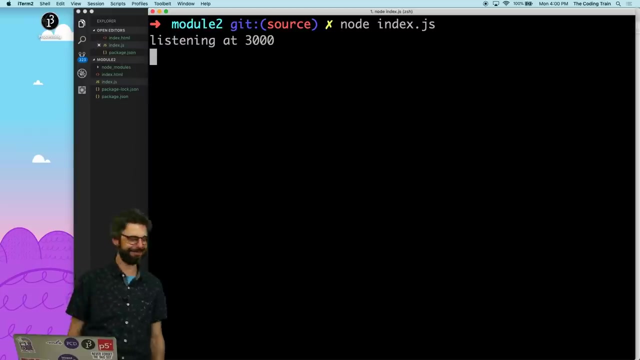 just say, listening at 3000.. There are nicer ways I could clean this up, but this is the idea. Require express, create the app and listen at a port. And there we go. I'm listening, I could connect, Should we connect? 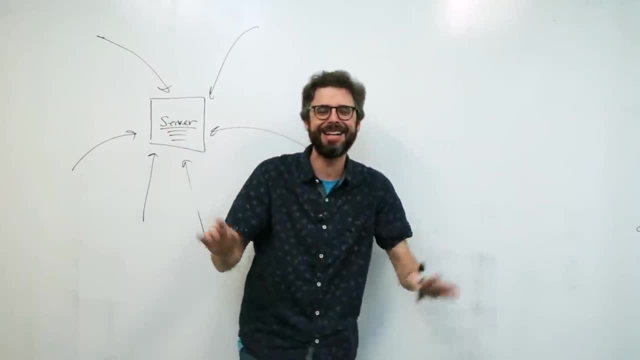 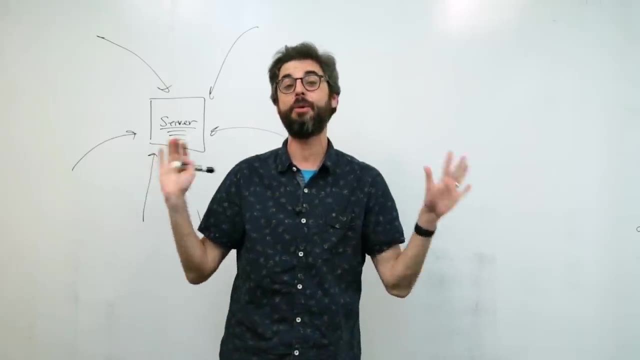 I'd be very happy to accept connections for 3000 right now, but I need to figure out: why am I here? what am I listening for? what kind of information am I going to send back? So let's make a list of some of the things I want the server to do, and it's pretty. 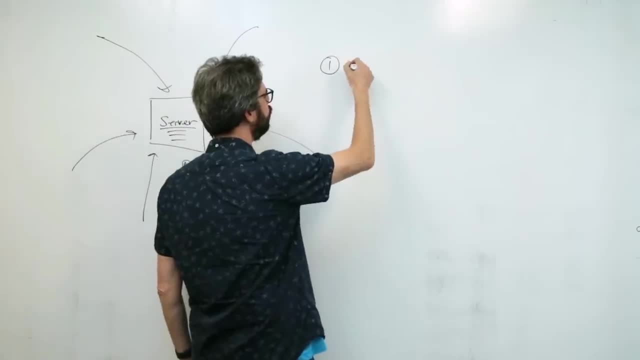 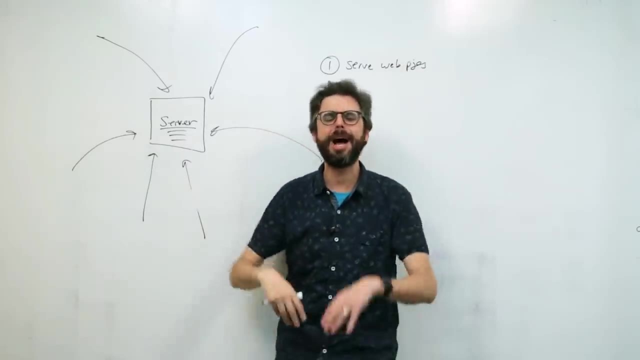 simple. for this app Number one, I want to serve web pages. In other words, right now I'm just a server running locally on this laptop at port 3000, but if I were to deploy my server to my website-thingy-urlcom? 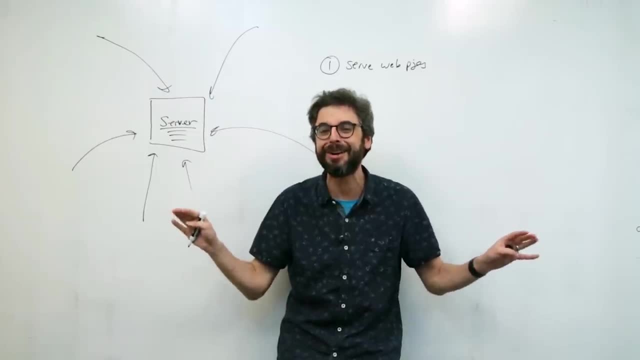 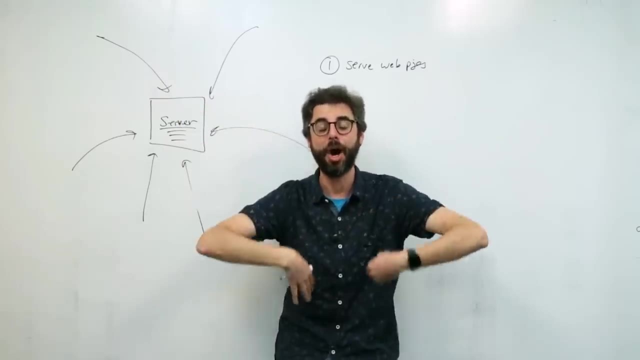 and people type that address into their browser. I want to send them the HTML and JavaScript and CSS and all that stuff that I have made for them to be able to see in their browser. So to simplify that, let's just serve one page: indexhtml. 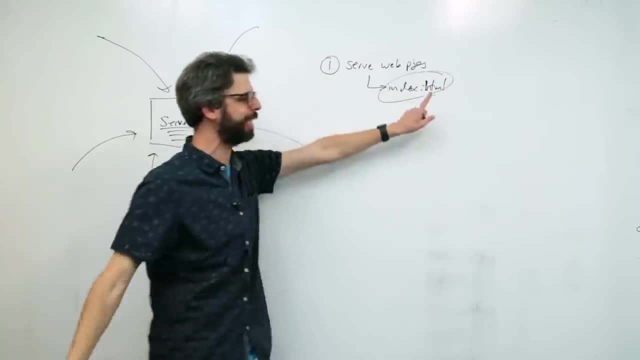 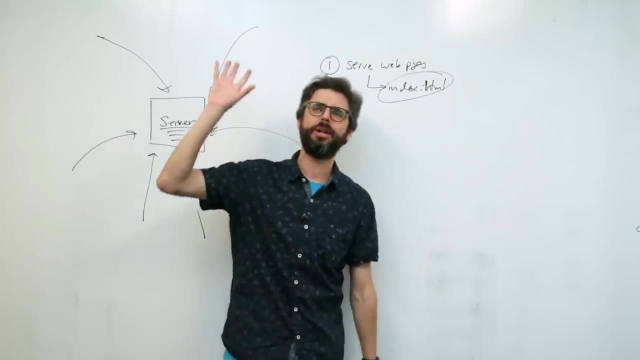 So when I open up my web browser, whatever content is in there I should see. So that's number one. There's other things that I want to do, of course, like I want to receive information and save it to the database, and then I want to be able to send information from the database. 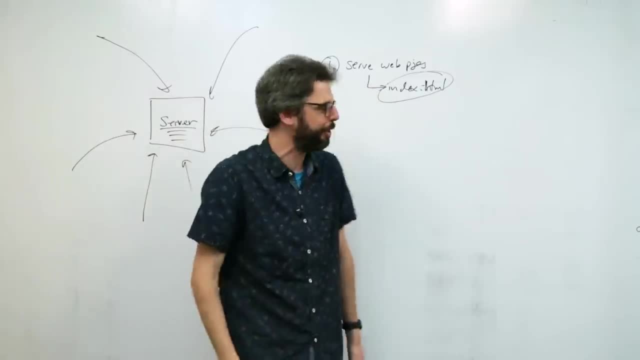 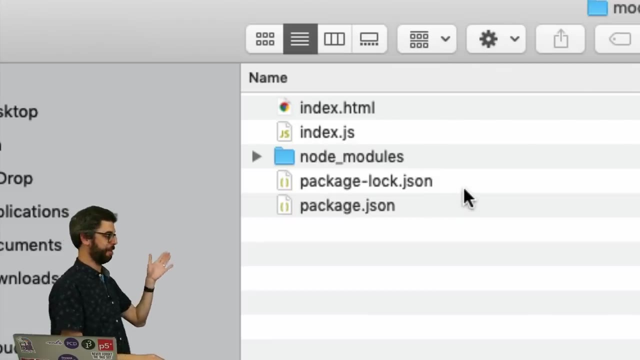 back out. but actually I'm going to get to that stuff as I go further and build this project. Let's actually just finish off this first part by serving a web page. So these are all the files I have already. I have packagejson. we know about that. 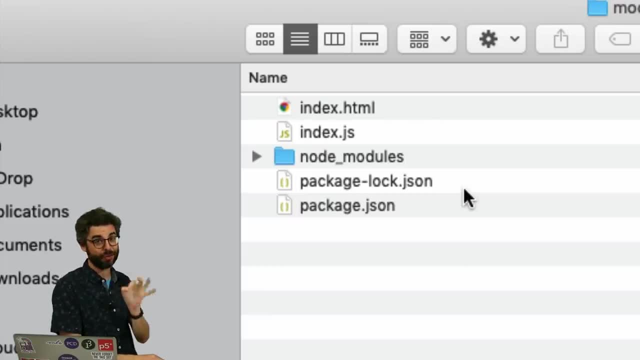 That's the configuration of my project. indexjs- that's my server code. This gets confusing because I want to have server code and client code. we've got to keep this stuff straight. I have node modules. that's all the node packages. 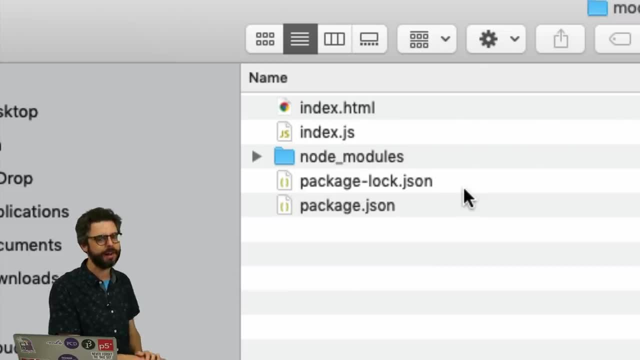 that I've installed. I don't need to look in there. There's also this package-lock file. it's kind of an important file. it's auto-generated, you don't need to touch it, but it's basically keeping track of the dependencies and versions. 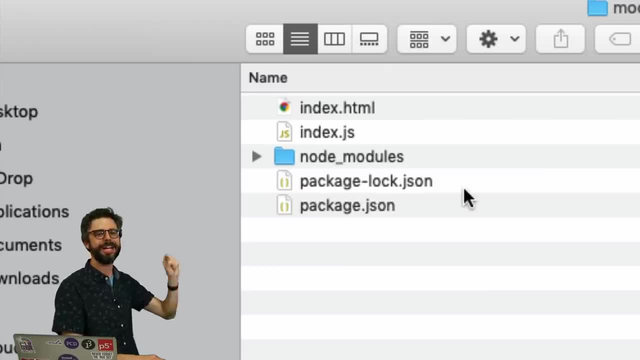 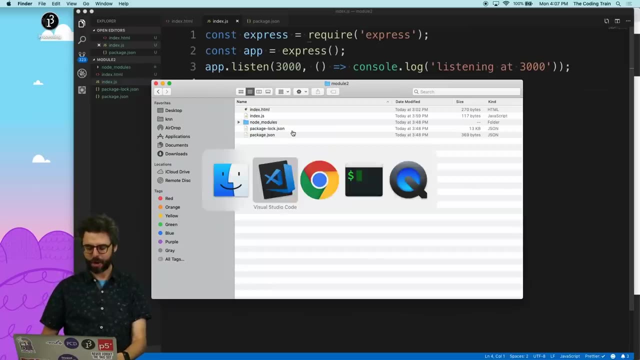 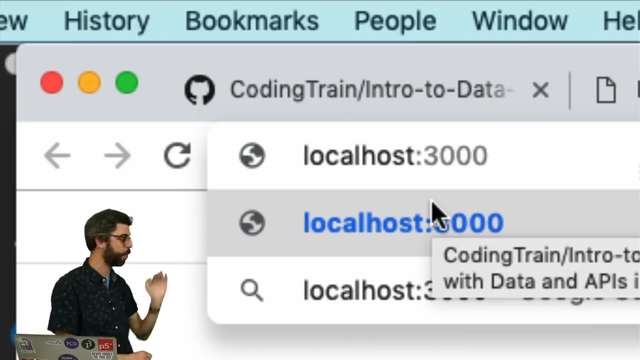 of your packages. Leave that aside. indexhtml: that's the file that I want to see. when I go and try to make a connection, Like right now, if I go to the browser and try to access localhost, that's my server running locally on this computer at port 3000. 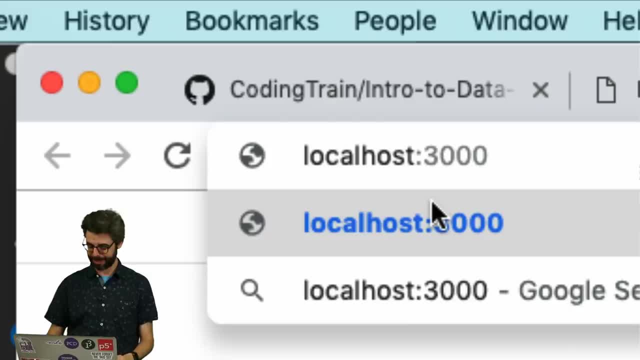 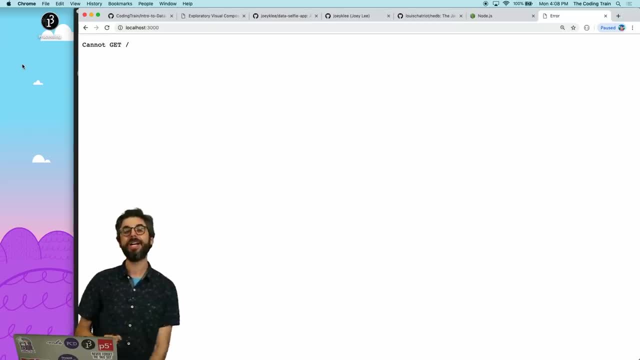 I should see whatever the server has and is able to give to me. So I hit enter and it can't get anything Because there's nothing there. I need to give it my indexhtml file, And the way that I can do that is by using 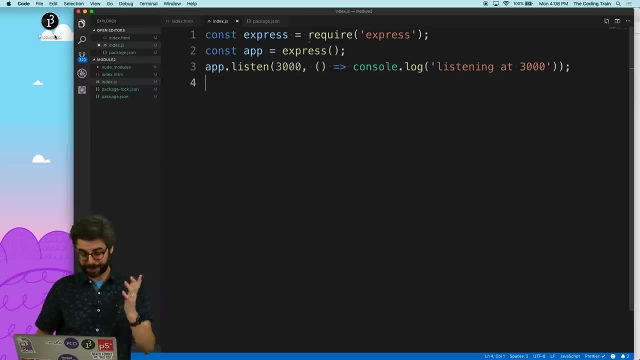 express to host static files. So what do I mean by that? First let me type it into the code. So I'm going to say appuse, I want to use expressstatic, and then what I need to give here is a directory name, or I could give one file. 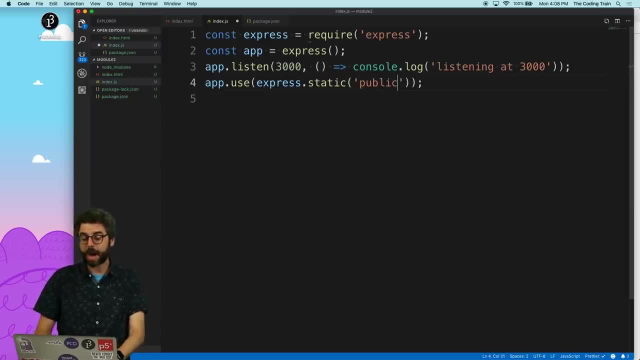 I might be able to say indexhtml, but better yet, I want to make up a folder name. Now I'm going to call it public, because I'm going to remind myself that anything that I put in that directory is publicly accessible from the URL, in this case, which is localhost. 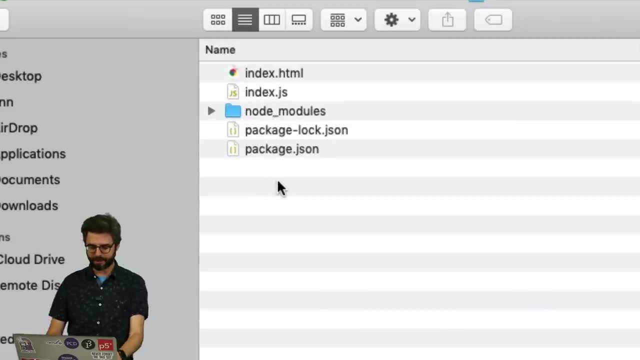 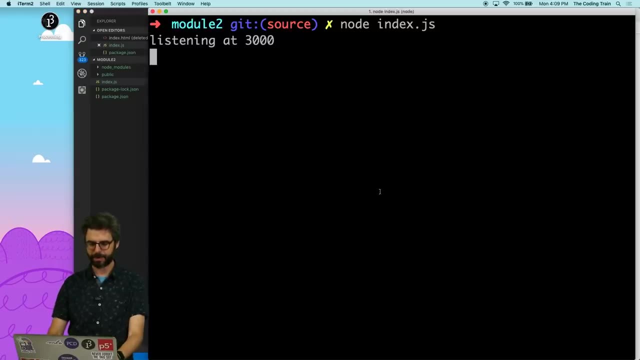 colon 3000.. So I'm going to go back to my finder and I'm going to make a folder, I'm going to call it public and I'm going to put indexhtml in there. So now, when I run this, I'm going to re-run my server. 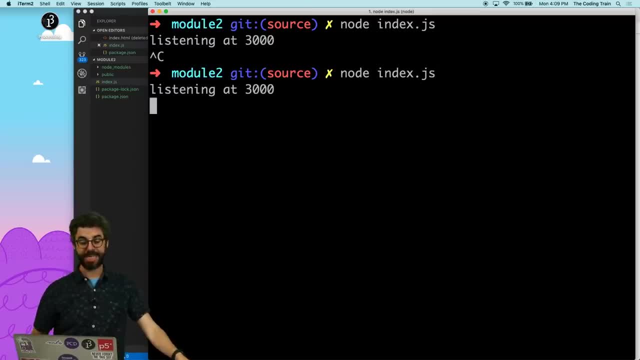 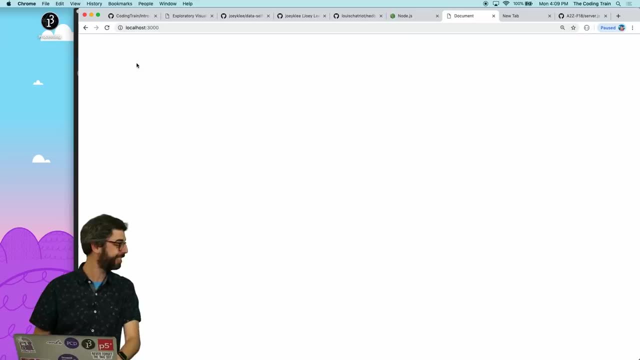 by saying node, indexjs, It's listening at port 3000. I go back and I refresh this page. it doesn't say it cannot get anymore. the problem is there's nothing there. well, it might be nice for me to actually add something to my indexhtml. 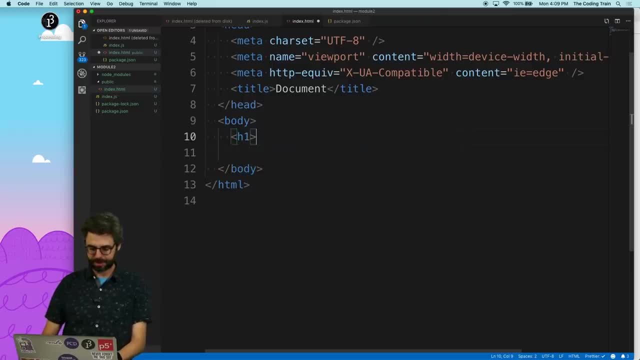 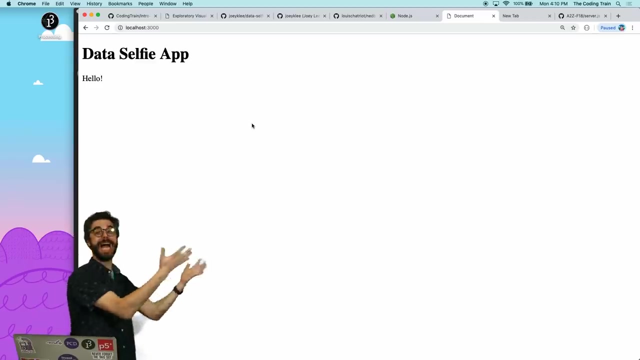 file, like I could say, data selfie app, add a paragraph hello, and I could start putting javascript in there and other things that we've seen so far, and now I'm going to hit refresh and there we go. I am serving up my web page Now. I haven't gotten that far. 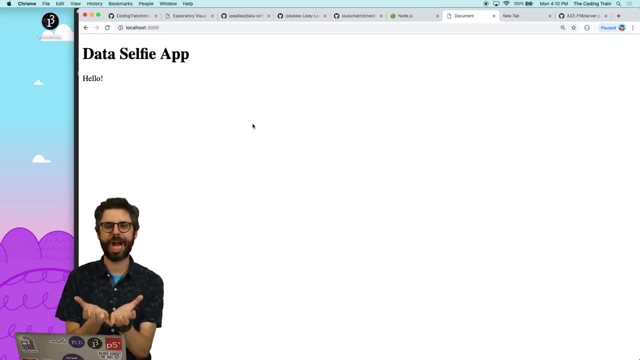 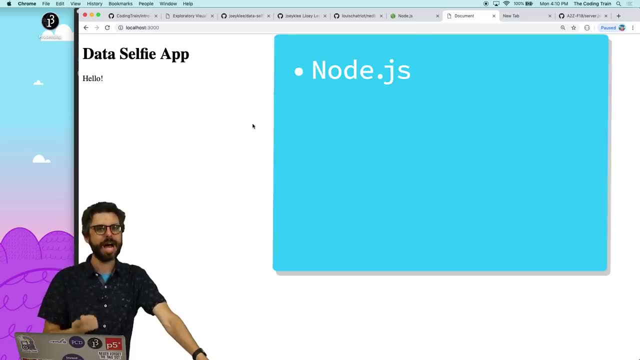 it might not seem we've gotten this far, but I'm really just setting up the foundation. I'm building the foundation for the house, this project that I'm going to build. what have I done so far? I've installed node, I've set up a project. 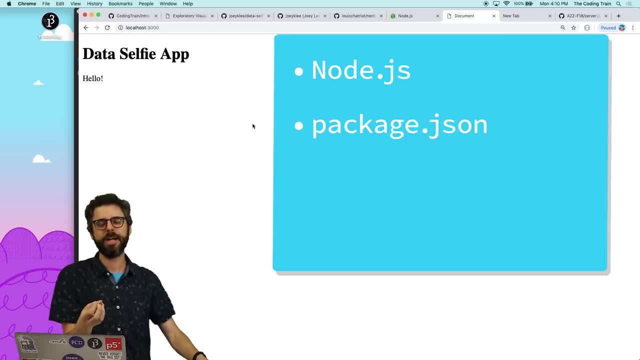 with npm init configuring a packagejson file. I've written a little bit of code inside an indexjs file using the node module express to create a web server, and that web server has one job. it has only one job: it's to serve up any files that are. 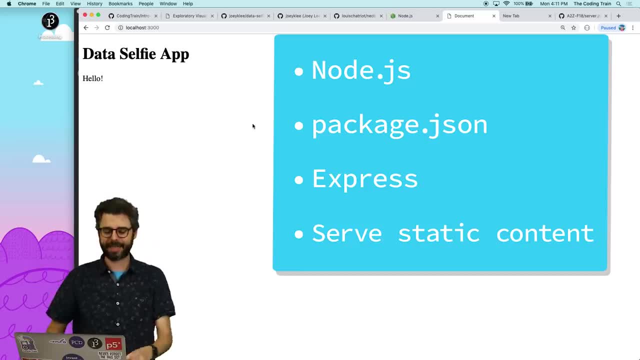 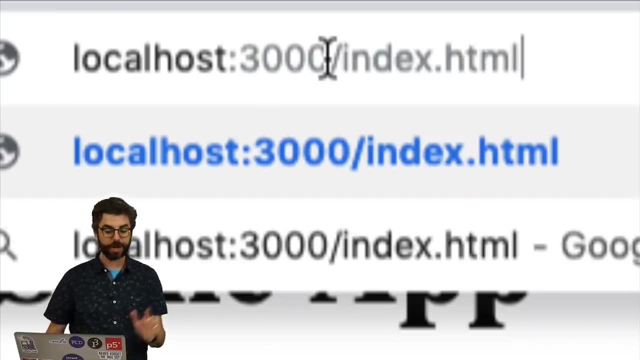 in the public folder, and the only file I have there right now is indexhtml. if I wanted to be really accurate about what's going on, I would type in indexhtml into the address bar itself, and now, when I hit enter, you see it's the same page. but I didn't have.